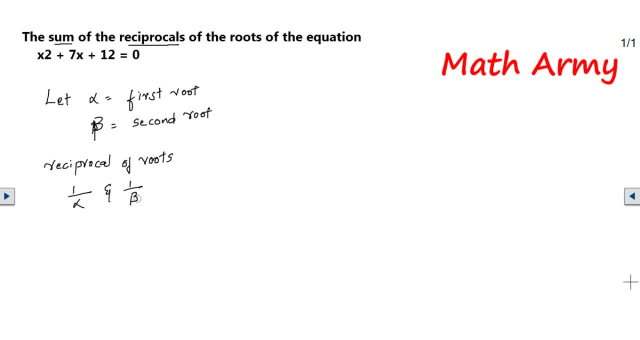 now. but what these people are asking in the equation sum of reciprocals. so add 1 by alpha plus 1 by beta is equal to 1 by alpha plus 1 by beta. guys, now alpha and beta are denominators, so do an lcm, obviously. 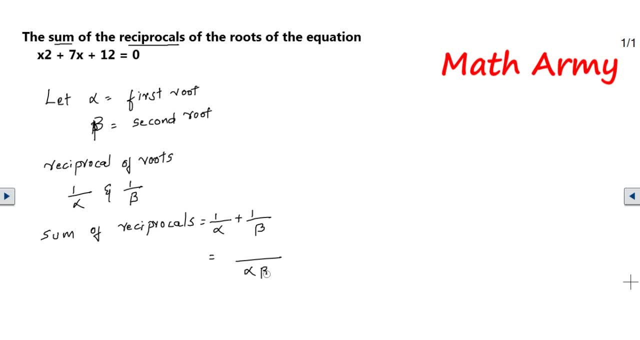 it will be alpha, beta. so at the numerator you will be getting beta plus alpha on solving. okay now, beta plus alpha can also be written as alpha plus beta. okay now, and the denominator is alpha, beta. now, guys, how the numerator is looking like. it is looking like an sum of roots, right? yes? 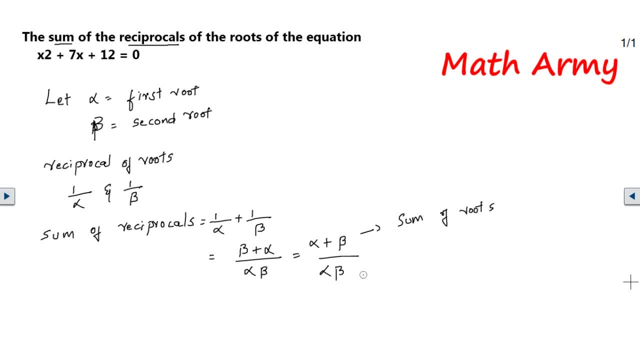 and alpha plus beta is looking like a sum of roots and alpha beta is nothing but product of the roots and everybody knows that. what is the formula for sum of roots? alpha plus beta is equal to what is the formula minus b by a right and alpha into beta, which is 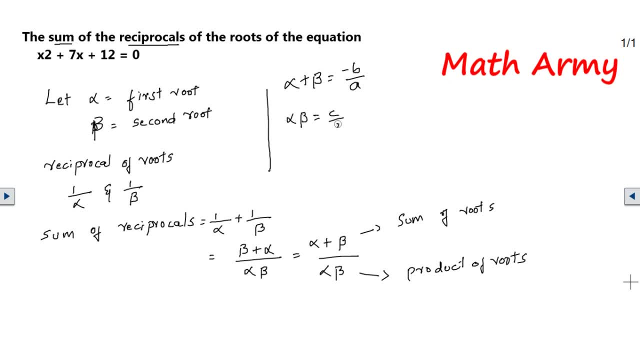 product of the root is c by a. okay now, what is the value of b? it is 7. so minus b means minus 7. divided by a, a value is coefficient of x square, which is 1, so minus 7 divided by 1 is minus 7. 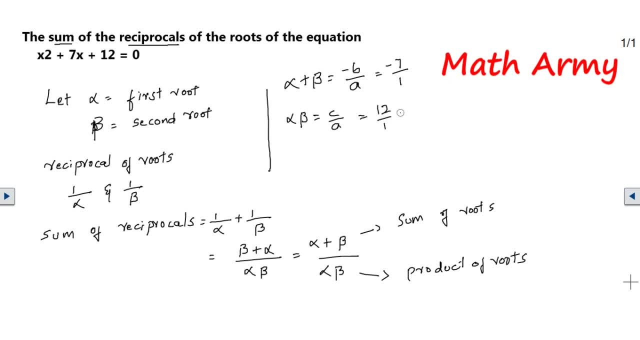 and c value is constant, 12 and a value is 1. now let us put these same values here: alpha plus beta. alpha plus beta is nothing but minus 7, and alpha into beta, which is product of which is 12. okay, and you got your answer. this is your final answer: minus 7 divided by 12. 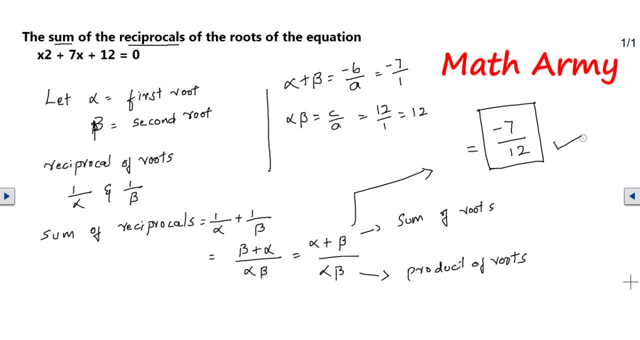 okay, so it is that easy. guys, don't get panic, and if you couldn't able to understand, just repeat. play it again. you will be understanding easily. and if you like my explanation, please don't forget to share and subscribe to my channel.